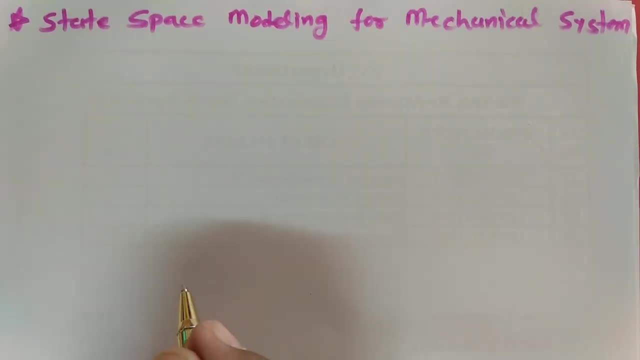 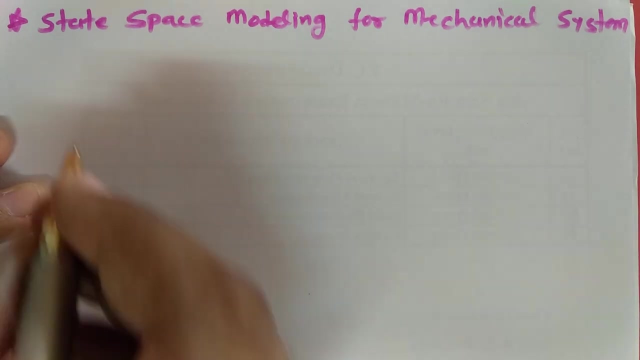 In this session I will be going to explain straight space modeling for mechanical system. So in previous session I have already explained few examples which were there with straight space modeling And we have identified advantages like multiple input, multiple output, which is there with straight space. 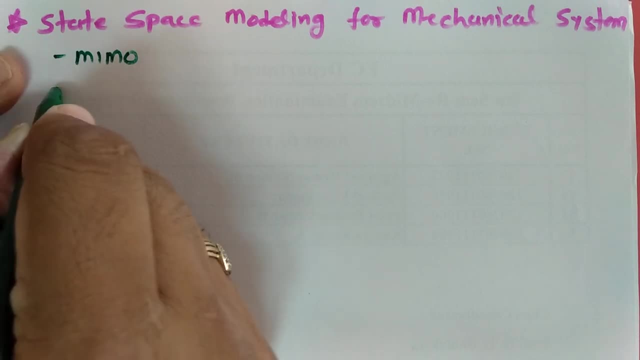 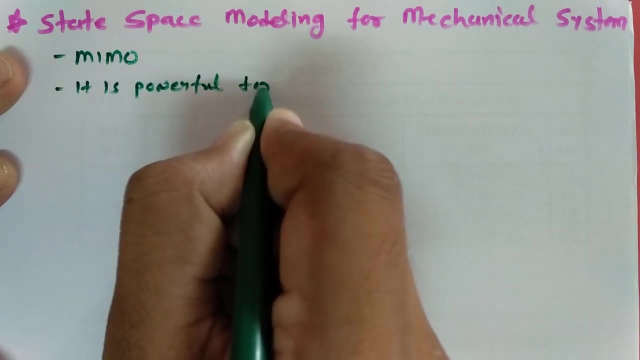 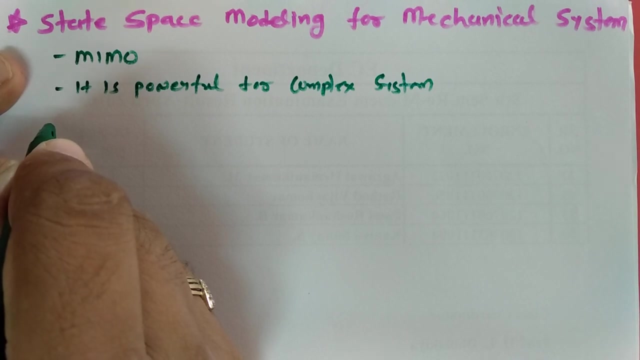 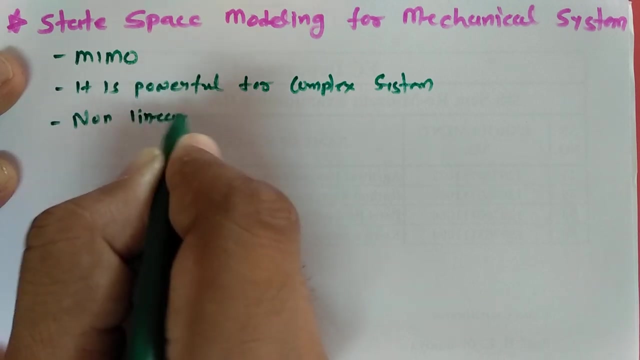 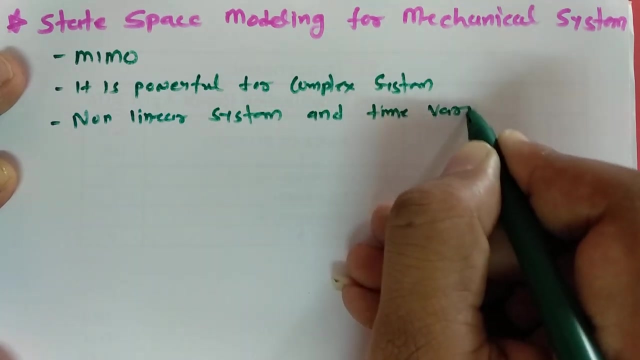 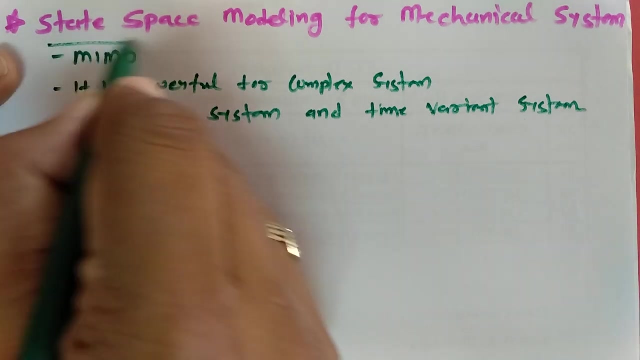 Straight space is so powerful system for complex system, So it is powerful for complex system And few more advantages that we have seen like it can work with non-linear system And time variant system. So these are few advantages, which is what we have seen for straight space modeling. 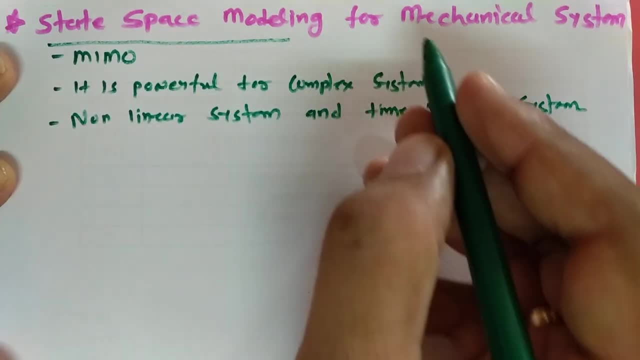 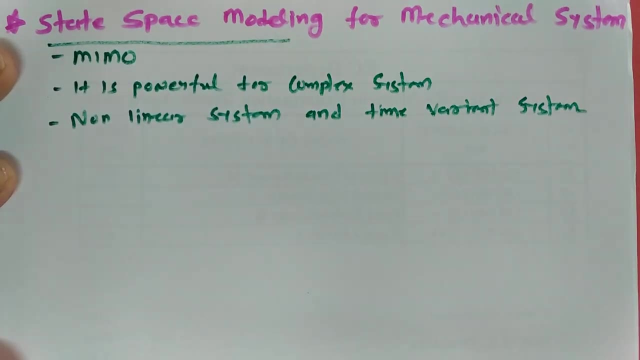 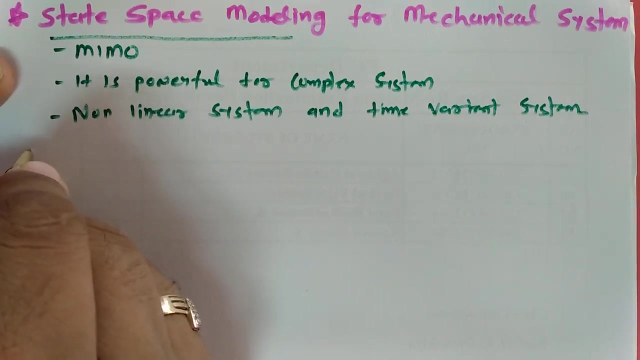 Now, in today's session, what I will be doing is I will be explaining mechanical systems modeling by using straight space. So let us have one example of mechanical system like I am considering right now, one example of spring. So if I consider a spring, 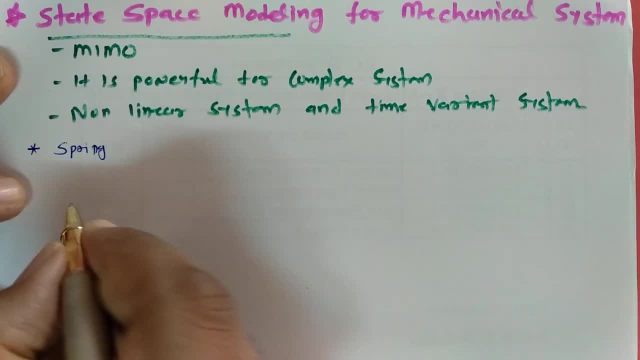 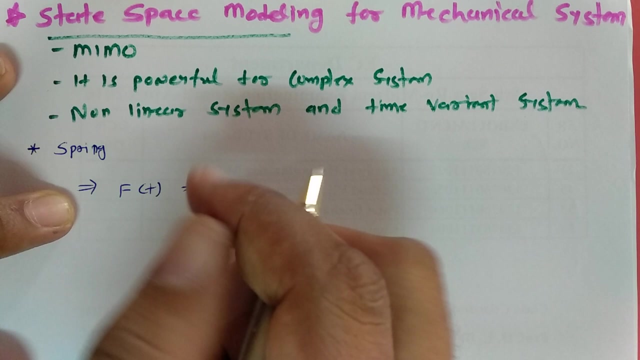 And if I give F amount Of force to this spring, Then what happens with that system is: let us give F amount of force, Ft, So that force that will get translated into acceleration And that force will get digested by spring. So let us have equation first and then I will explain what are those terms. 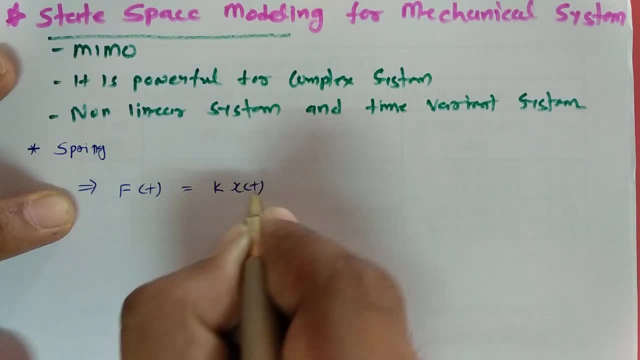 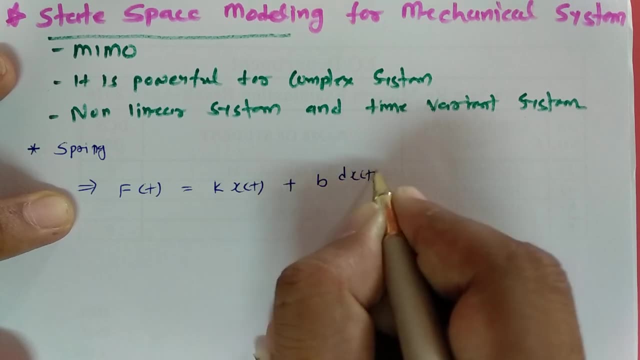 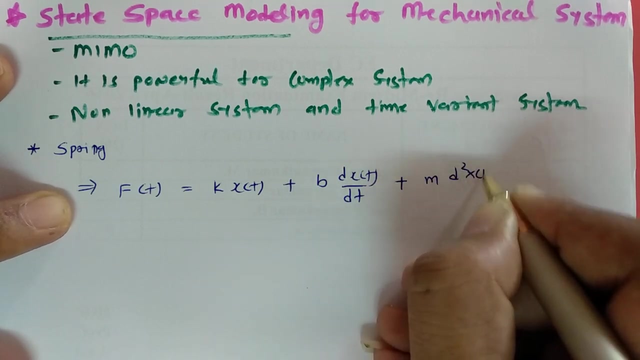 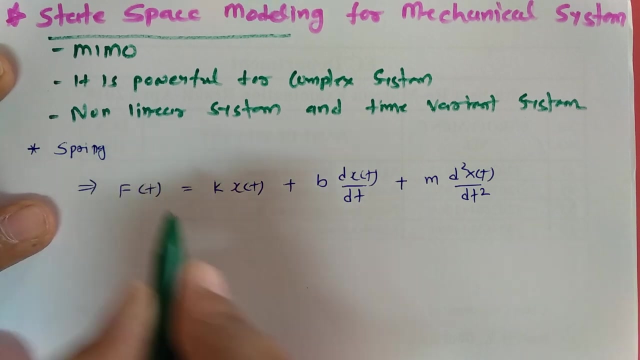 So that force will be K into Xt plus if resistive force that is there with resistive constant B Into d, Xt by dt plus mass into acceleration, that is d square, Xt by dt square. So here if we see this spring example in which this force that is related to spring, 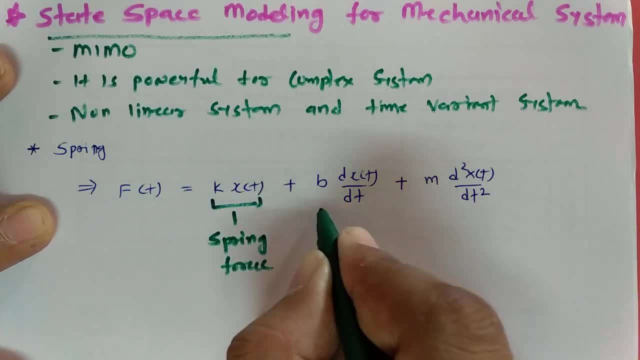 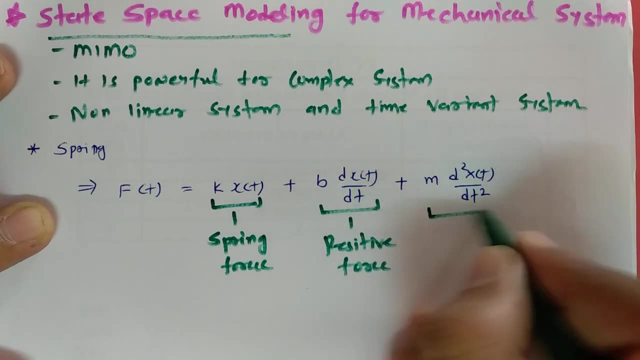 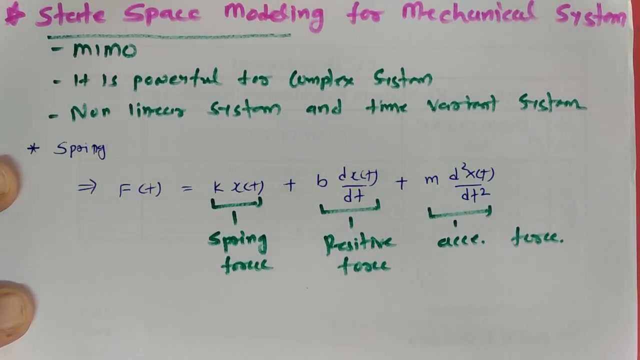 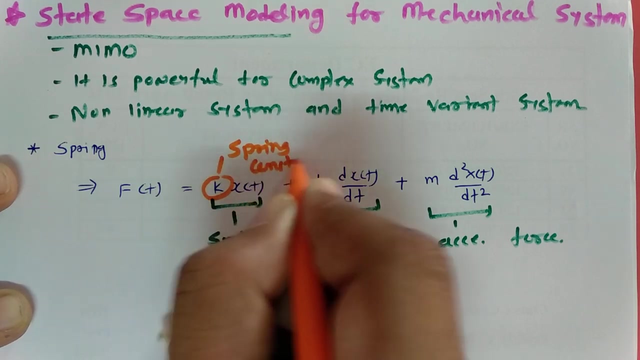 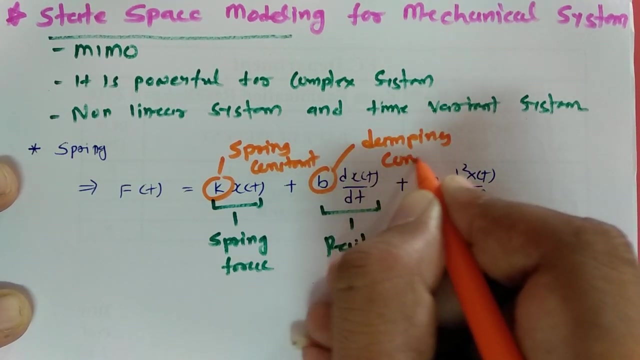 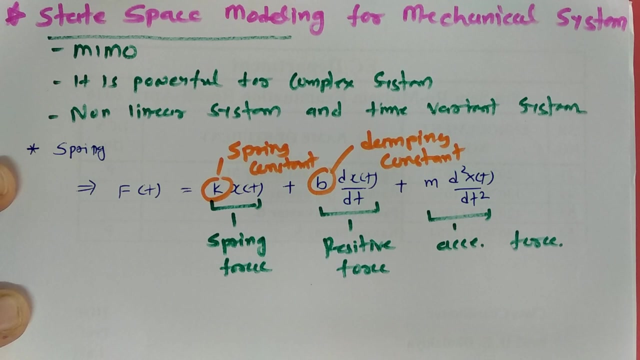 So this is spring force, This is resistive force And this is accelerative force. So here this is accelerative force And one can see this is spring constant, This is damping constant And this is mass. So that is how this spring is a system, which is what we have considered. 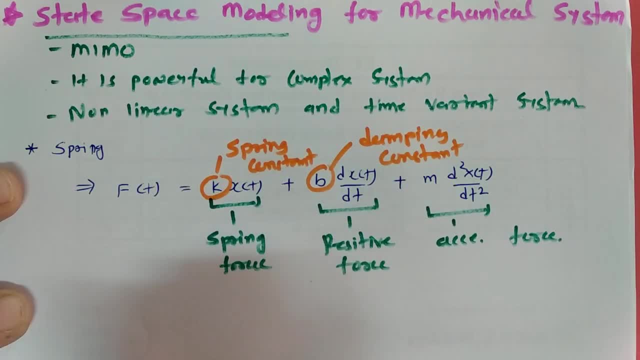 Now in this session, I will be explaining state space modeling for this. So here, before I do all those things, let us try to understand those terms which is there in this very simply, And then at the end, you will be able to understand how things are happening inside. 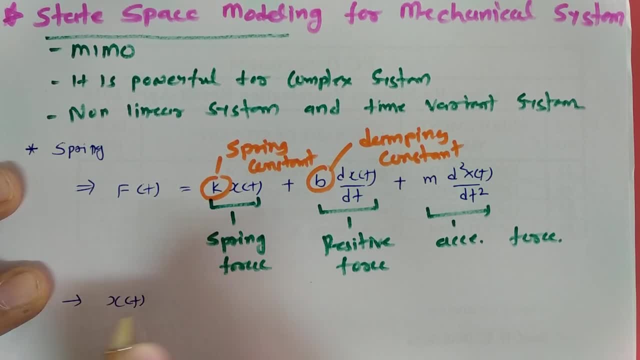 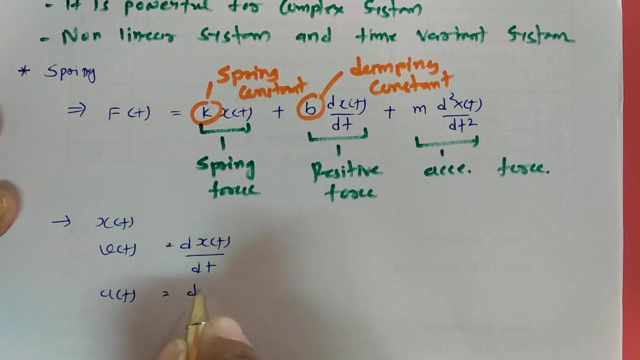 So here Xt, that is what distance, Here Vt, that is velocity. So that is differentiation of Xt with respect to time. Here acceleration, that is change in velocity with respect to time. Now, before I place that into state space variable, let us consider few variables. 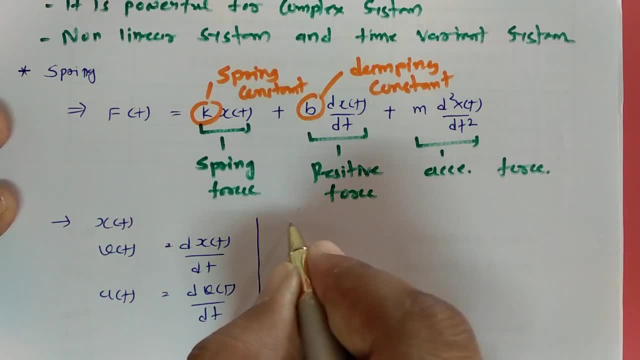 So if I consider State space variable over here in this terms, So state space variable that I am considering, So let us say Xt, that is distance. Let us consider: this is what X1. I am just considering variable. So one can say: this is what Vt, that is differentiation of Xt with respect to time. 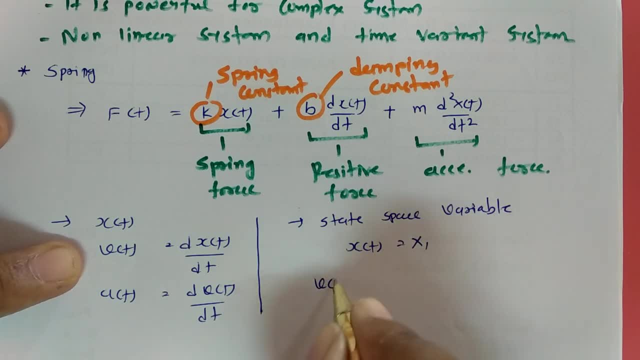 So Vt, that is actually differentiation of Xt with respect to time. So one can say: this is what X1. Dot means: it is differentiation with respect to time And let us consider that as a variable to X2.. So based on this, one can say X2 dot, that will be differentiation of velocity with respect to time. 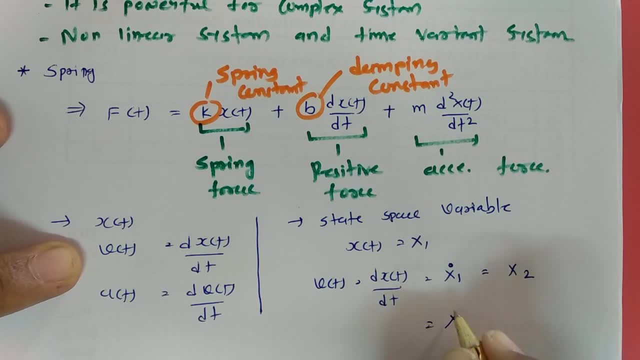 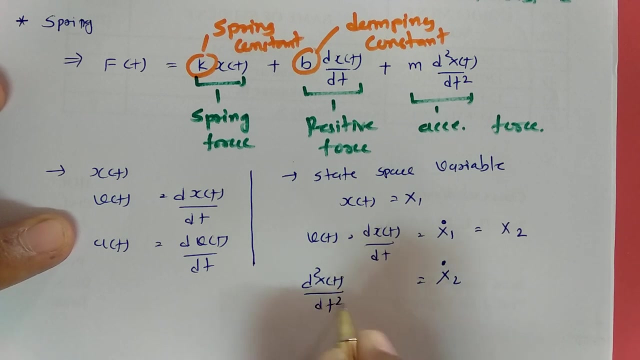 So from this one can say: this is what X2 dot, And that will be double differentiation of this. or one can say that is what dx2 by dt. So this is even called as d square, Xt by dt square, or that could be even said as dx2 by dt. 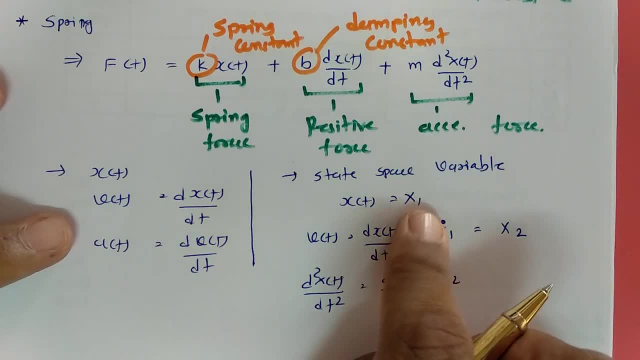 So here I am considering just two variables. One is X1, that is distance, and second is X2, that is velocity. So acceleration will be differentiation of X2 with respect to time. So here I am considering two variable: X1 and X2.. 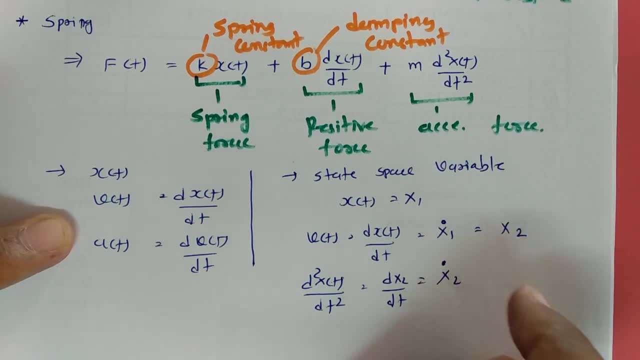 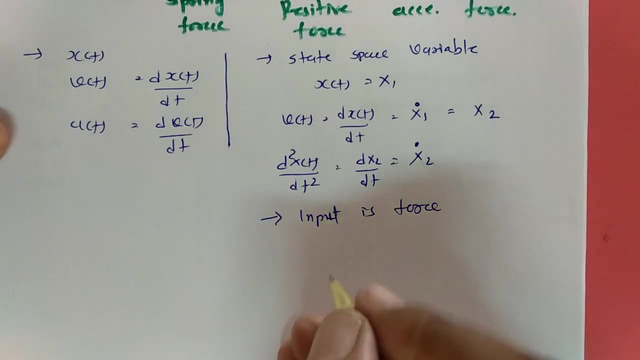 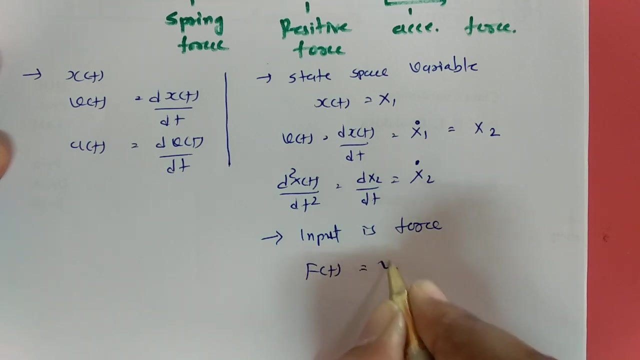 And this two variable that I will be going to use that in state space variable. Now here I am considering input, that is force. So input is force. So here Ft that I am saying like It is U1.. Ft is U1.. 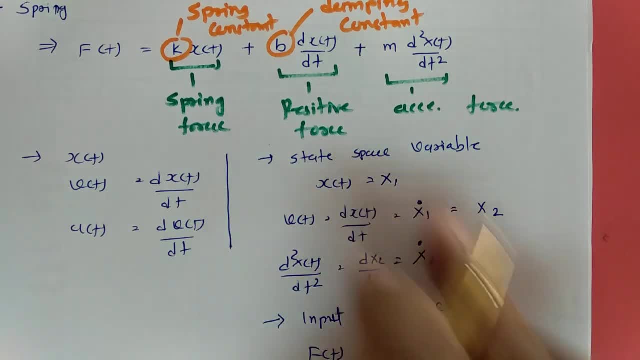 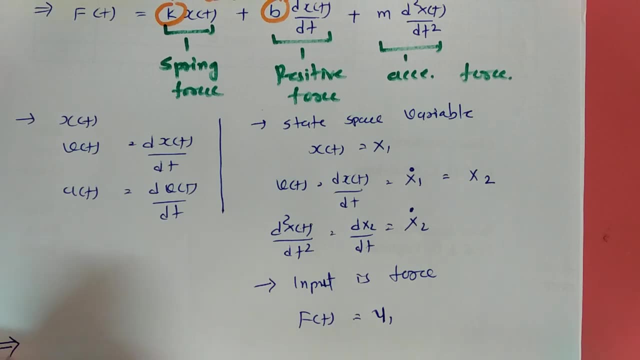 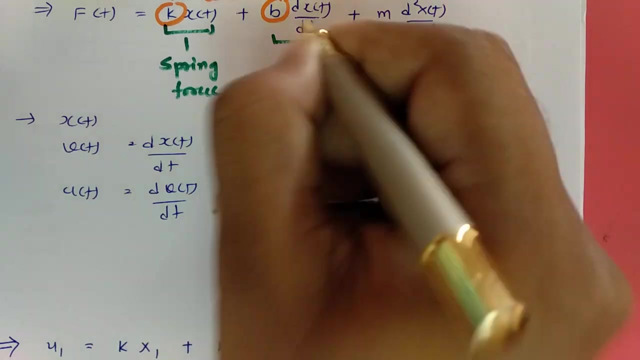 So now let us have this equation again in terms of state space variables. So Ft, this Ft that will be U1 is equals to This, will be K into X1.. Plus B, dx2 by dt, that is velocity. So that is what actually X2.. 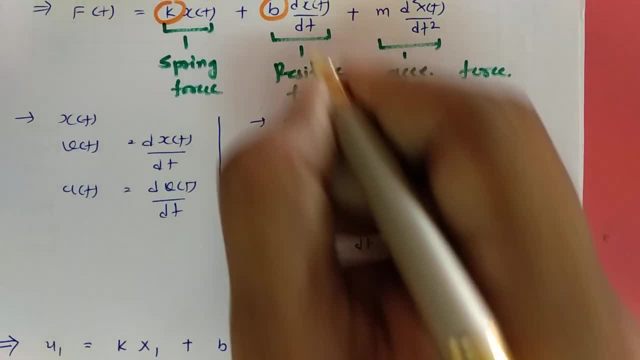 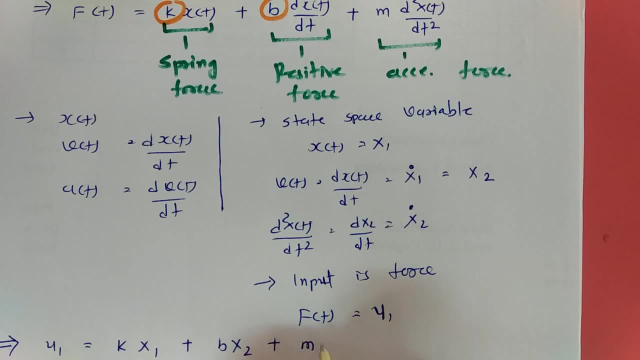 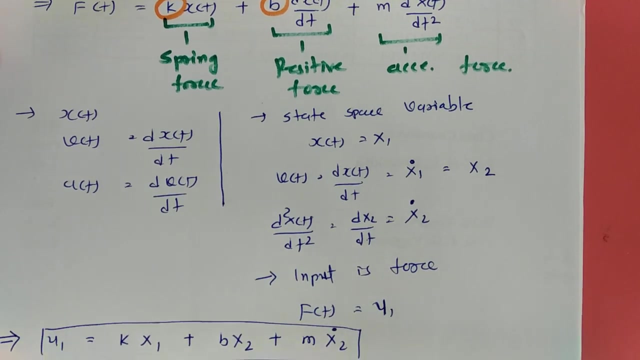 So BX2 plus M into d square, Xt by dt square, one can say that is X2 dot. So this will be M into X2 dot. So this is what equation, which is what I am having right now. Now my aim is to translate this equation in terms of state space matrix. 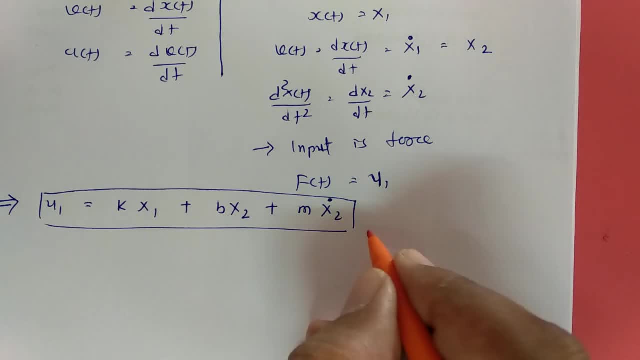 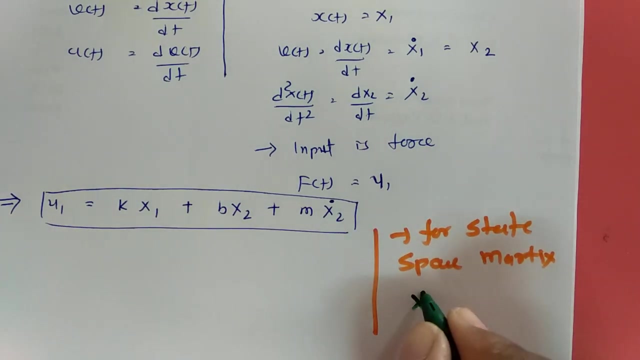 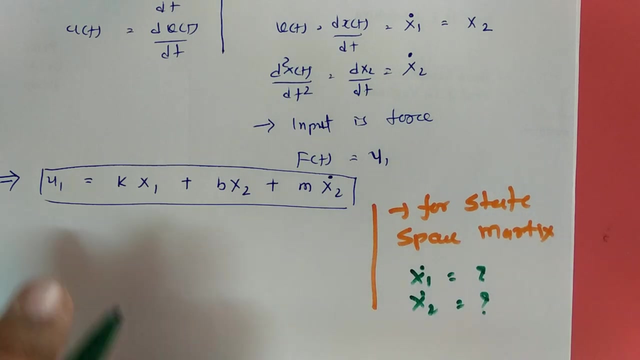 And when we wanted to have state space matrix. So for state space matrix, I need equations in terms of X1 bar and X2 bar. So this is what I wanted to have. actually Now to have this, what I will be doing. 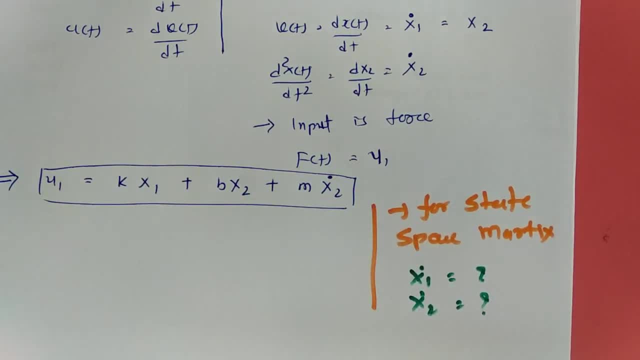 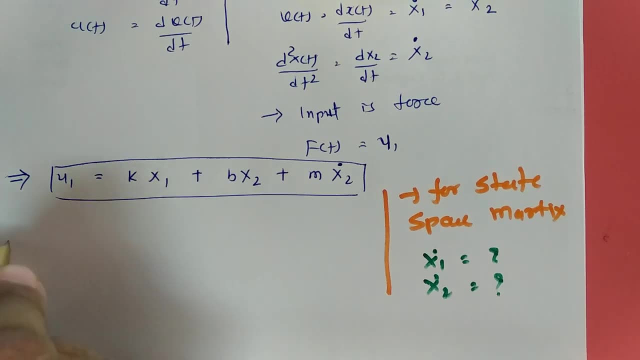 I will be translating this equation in terms of X2 bar. So here To have this state space matrix equation. Let us translate this equation in terms of X2 bar. So one can say: X2 bar, that will be U1 by M into U1. 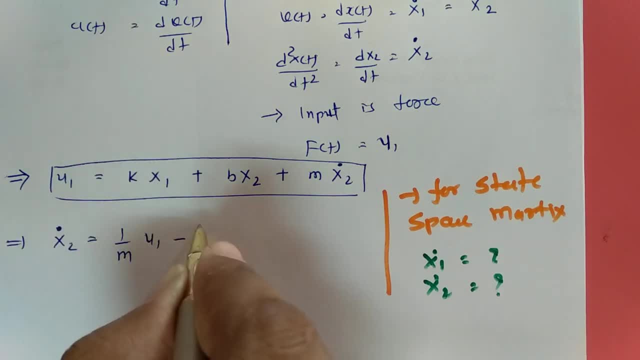 And take this over this side, So that will be minus K by M into X1.. And even this will be over, this side will be negative, So that will be minus B by M into X2.. Let us rearrange this. 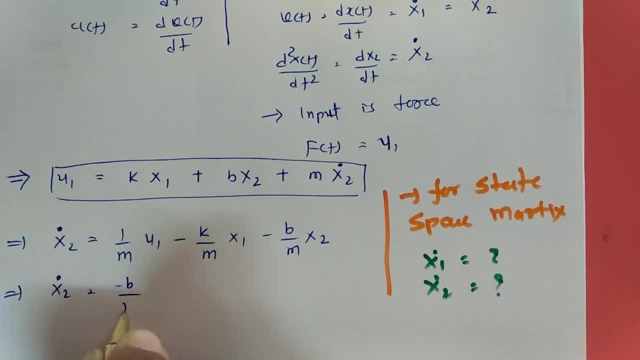 So X2 bar, that will be minus K by M X1, minus B by M X2, plus 1 by M U1.. So this is what one term, which is what I am having Now. similarly, I can write X1's equation: 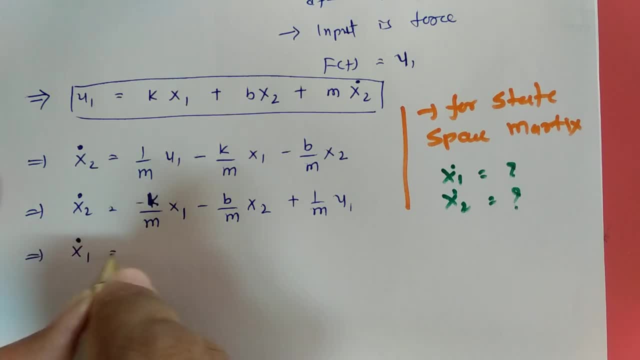 X1 bar's equation. So X1 bar, that will be actually X2.. So let us rewrite this equation in similar form So that we can have matrix form. So X1 dot or bar, So that will be X1 into 0.. 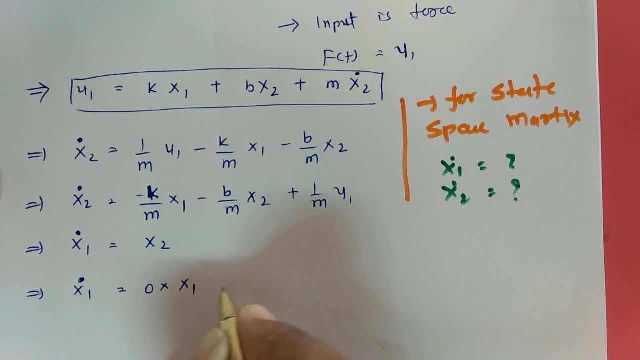 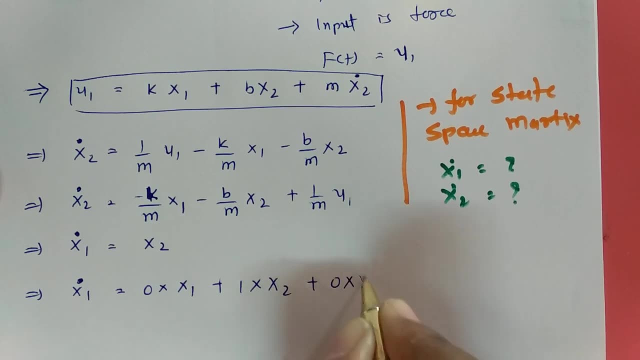 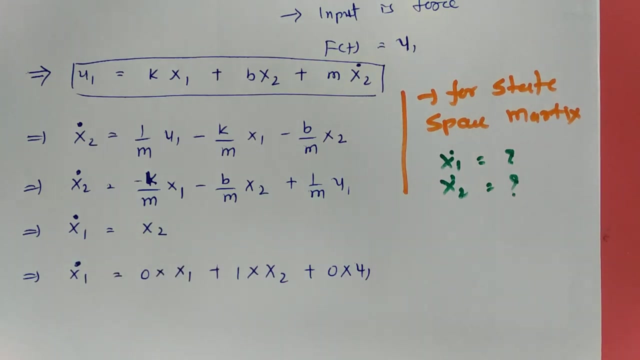 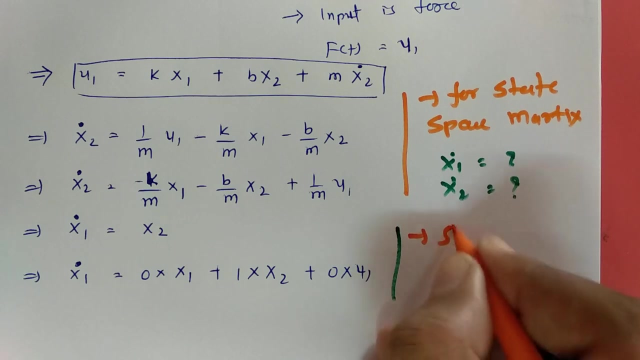 So 0 into X1. Plus 1 into X2. Plus 0 into U1.. So that is how it is there. So if I want to write state space equation, So state space equation, State space equation- that is there in matrix form as per. 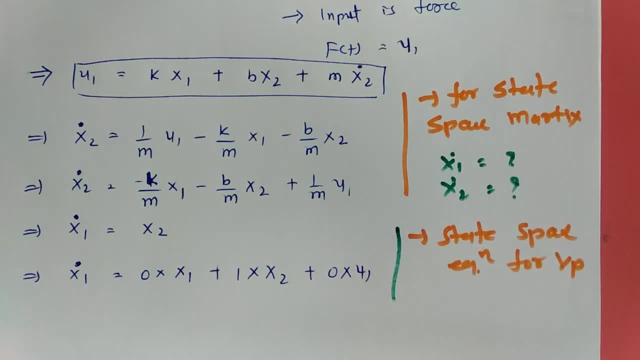 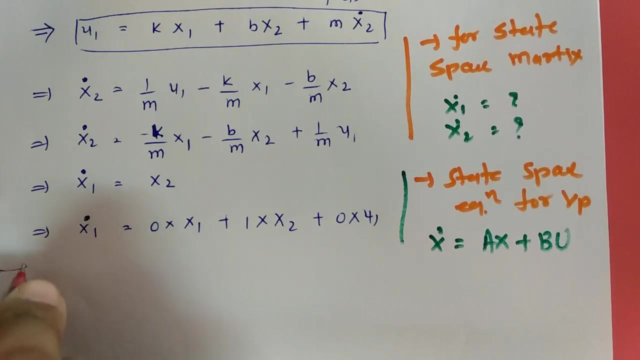 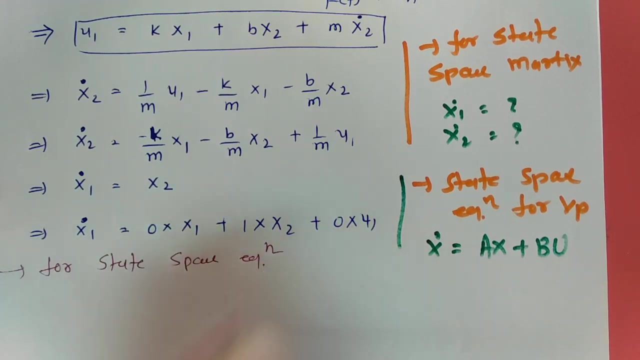 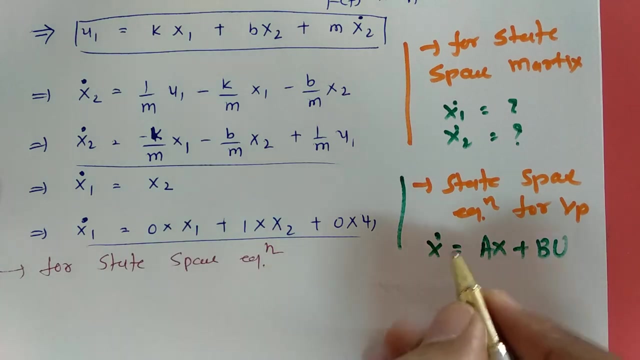 For input, That will be X bar is equals to AX plus BU. So this is what the form which I wanted to have. So, for state space equation, For state space equation, Let us have this: two equations And that will be resulting into state space equation in this form. 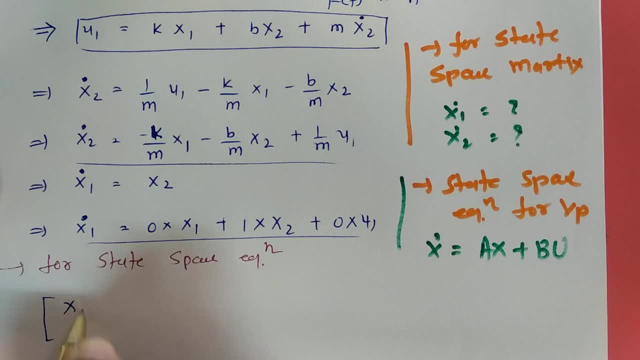 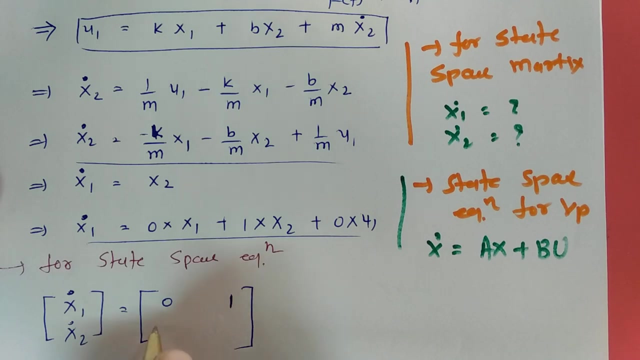 So that will be X1 dot, X2 dot in matrix. And now, as per this term, I will be having this matrix by. This term is 0.. This term is 1.. And this term is minus K by M And this term is minus B by M. 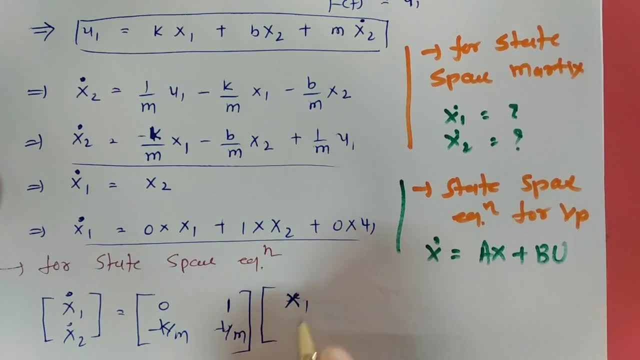 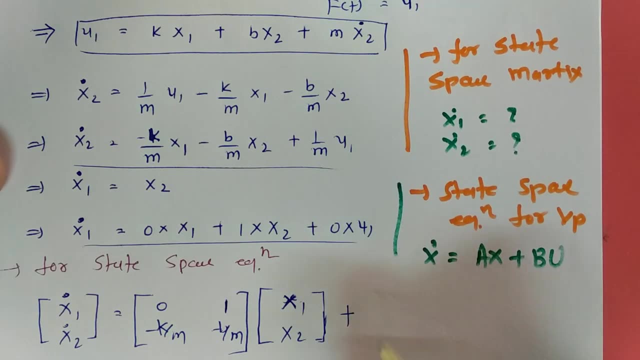 AC. Yeah, So this is where is zero ного. 1 by 1 into AX1. X2 plus X1 is must bigger than 2.. Here you have amax minus 12.. What you just wrote out here, that is a matrix. 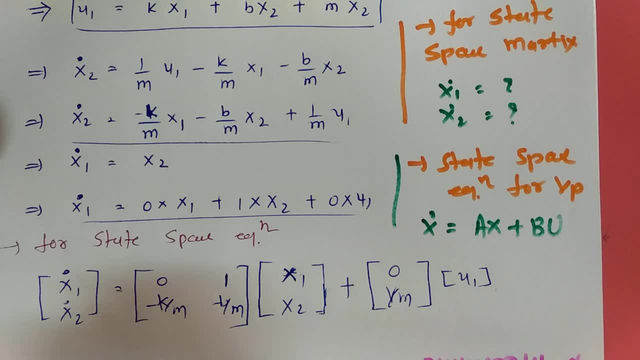 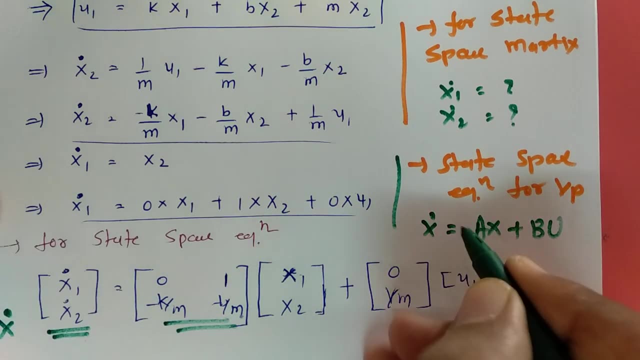 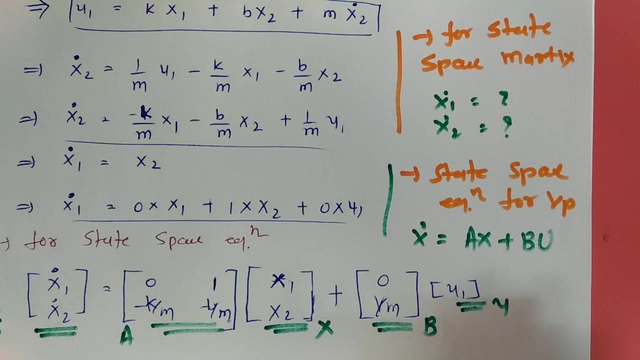 So now, So you have AX- only two paper- inside, And you have this Bia and this Bia. So that means: So this one is und 분, this is what matrix a, this is what matrix x, this is what matrix b and this is matrix u. so this is how one can translate. 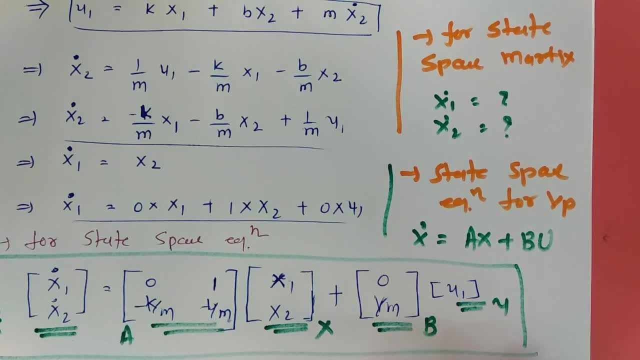 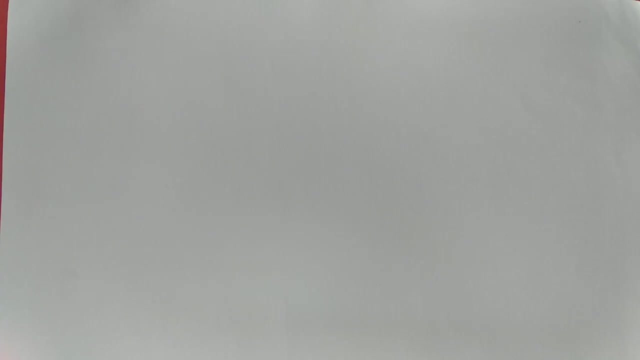 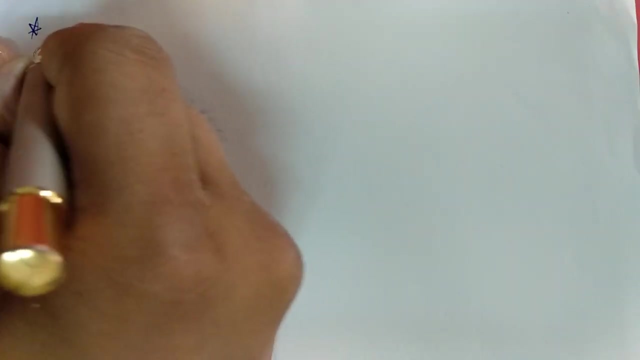 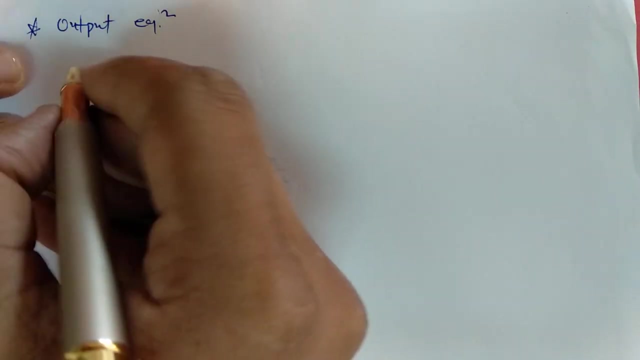 state space input equation from mechanical system. and this is what having this form, which is as per x blot, is, equals to ax plus b. now let us have output equation. so output equation for state space matrix. so for that. so before we derive output equation, one should have basic idea about what should be output. 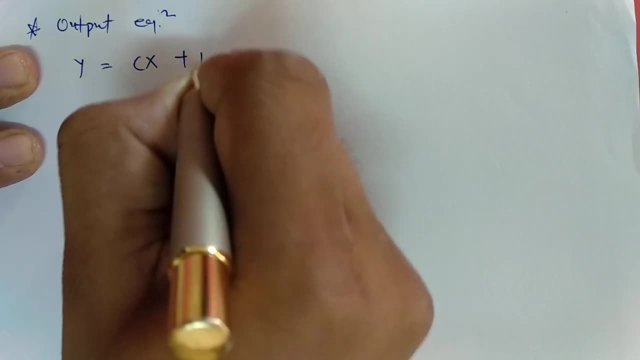 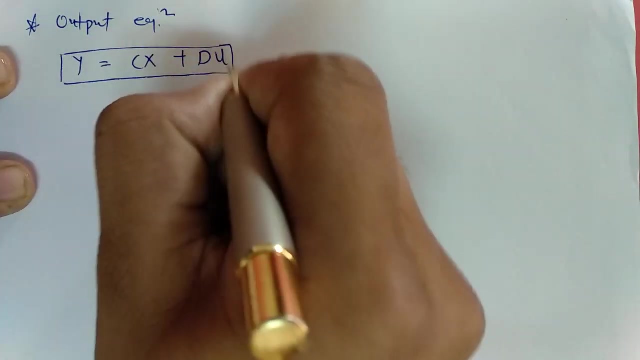 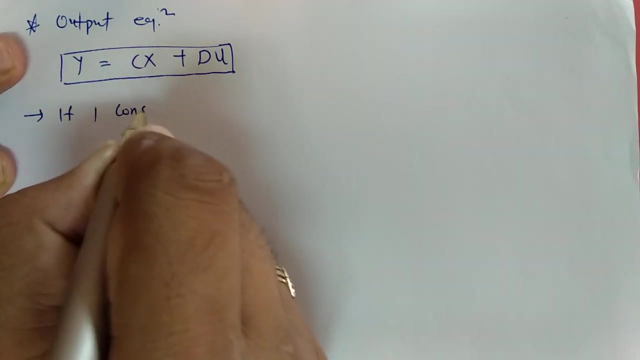 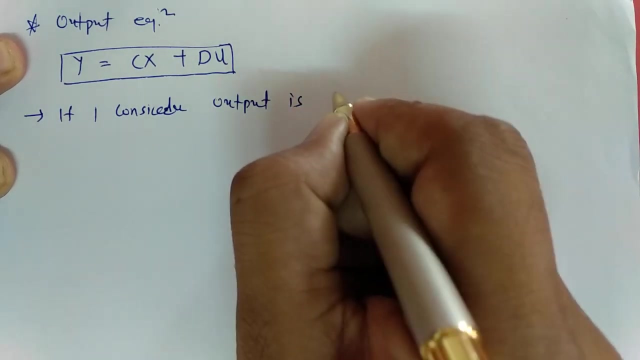 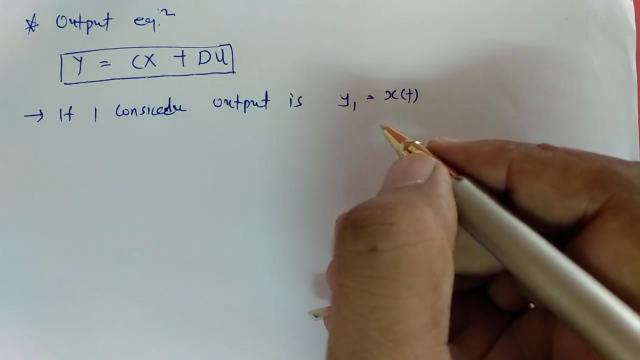 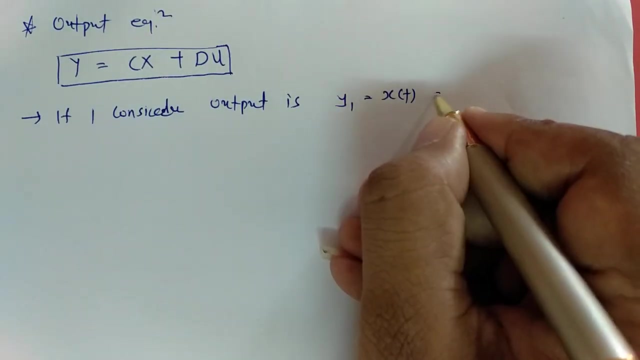 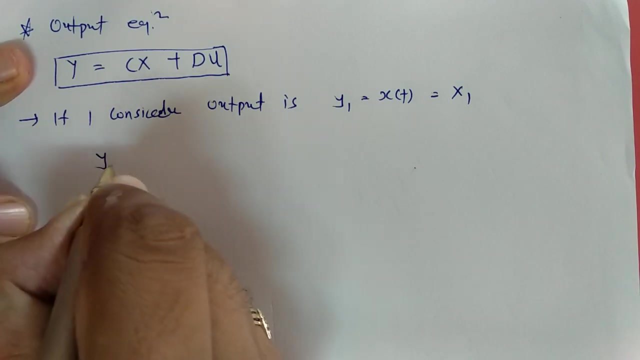 equation. so output equation should be cx, cx, cx, cx plus du in terms of matrix. so this should be output equation. now, if i consider my output is distance, if i consider output is y1 is equals to xt and in this question i have considered x1 as xt. so this is what output which is actually x1. so my output y- let us say y1. 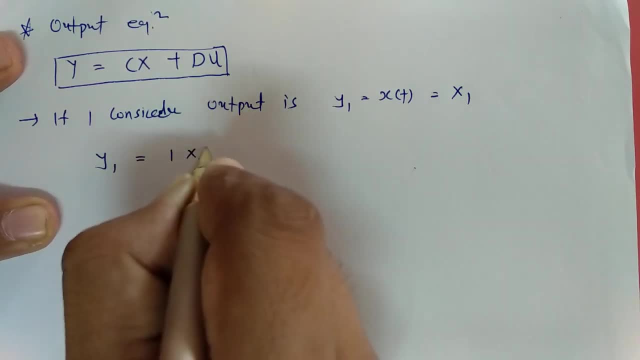 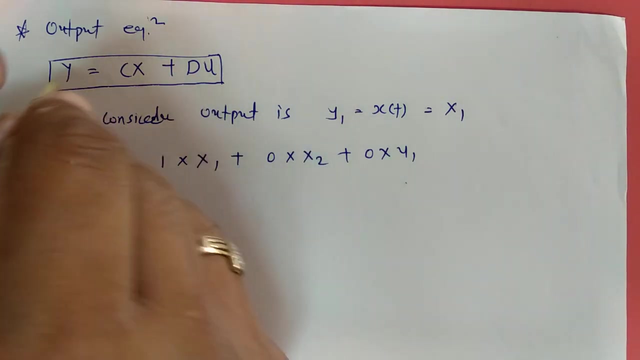 so that will be 1 into x1 plus 0 into x2 plus 0 into u1. so that is how my output will be there. so, based on that- so basically i am saying here function- i have found this formula that from this matrix and 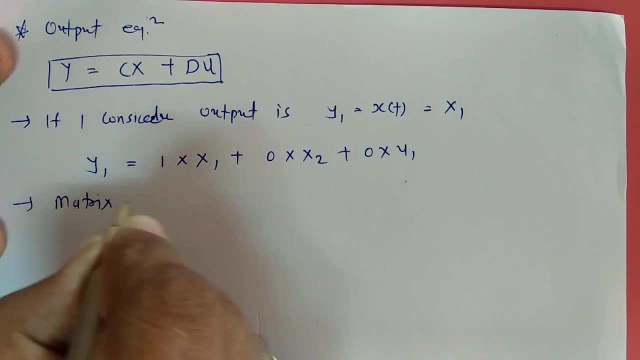 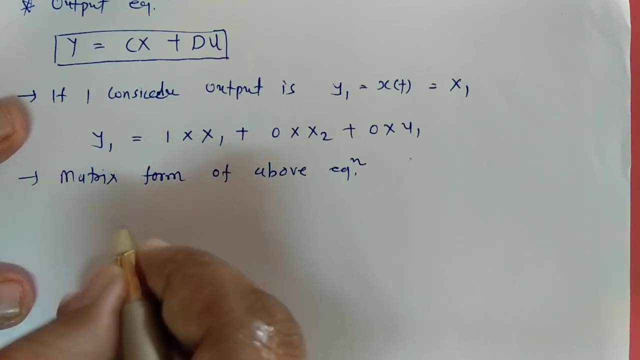 this will be the time najwię sub Roberto Gibbs et al by x1 and x2. so if i say x1 is 0 here, then I am going to get� Strawberry этиc of above equation and matrix form of above equation. now that will be. this is what y1 is equals to. these are having variable one and zero. so I am writing 1 and zero and x1, x2. that is result if these two, Nicholas W, actually xt. so I am writing 1 and 0 and x1 and xt. 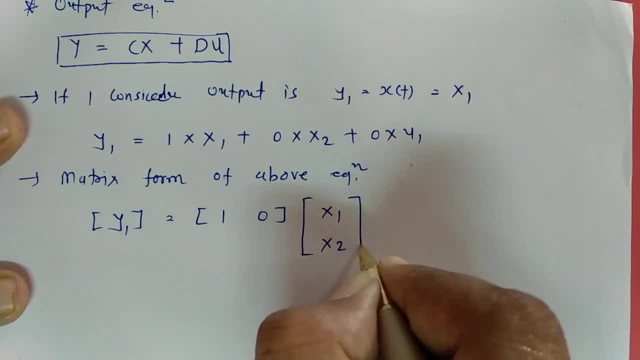 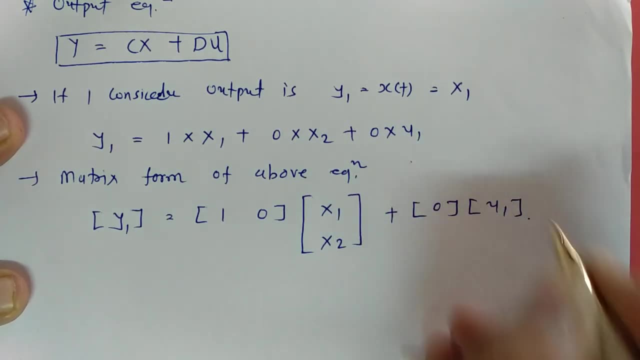 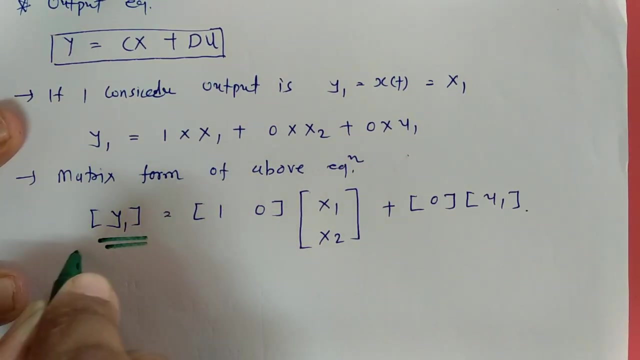 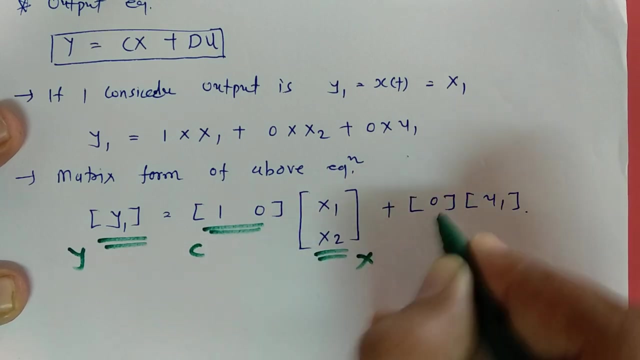 is as this: x1 and x2 plus d matrix, that is 0, and this is what u1, which is input. So that is how I can write this. So here one can say: this is output matrix y, this is c matrix, this is x matrix, this is d matrix and this is input matrix. So that is how it is there and this. 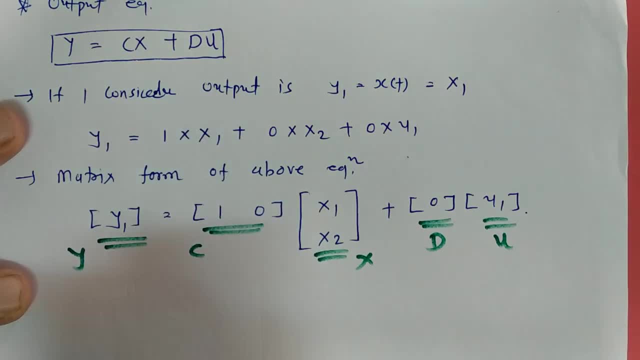 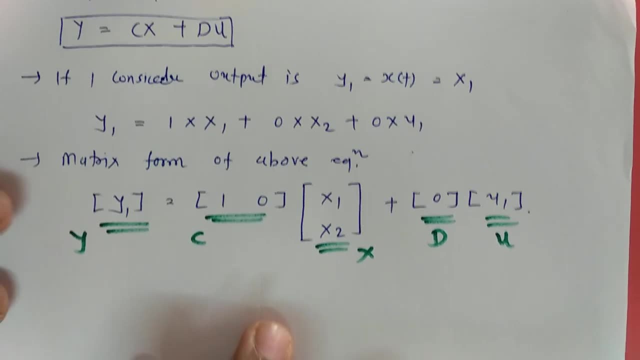 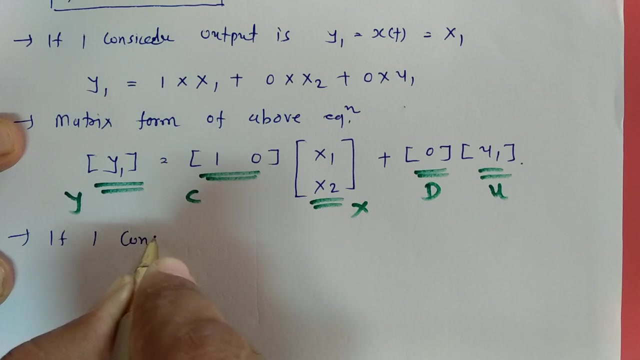 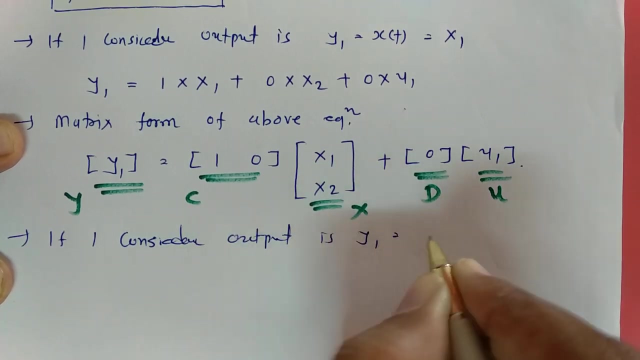 is what there in terms of y is equals to cx plus du form. Now if I say: my output is velocity, even then we can write same equation. So let us consider first if I say: if I consider output is y1 is equals to velocity, and that is actually dxt by dt, and that is actually x2, which is: 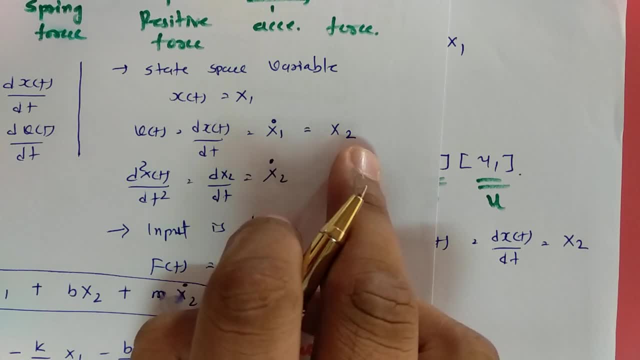 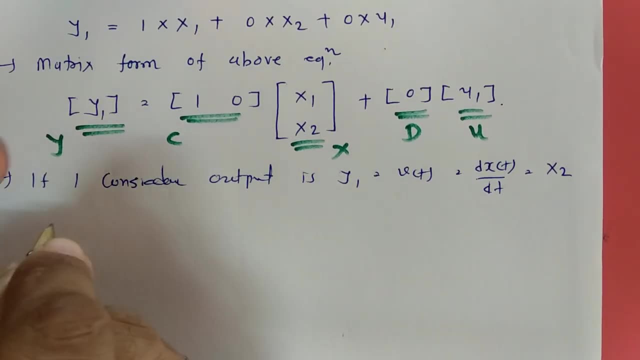 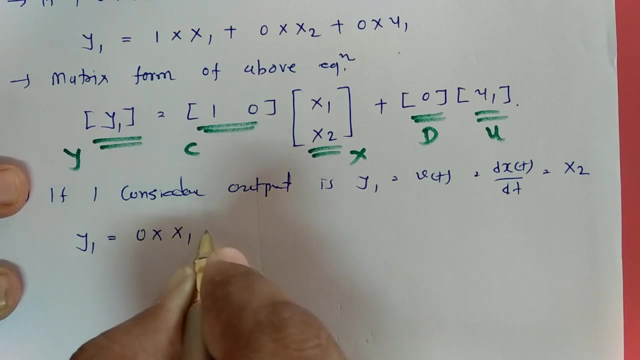 what we have considered. x2 is equals to dxt by dt. So now my equation will be: y1 is equals to 0 into x1. Plus 1 into x2, plus 0 into u1.. Now let us translate that in a matrix form. So matrix. 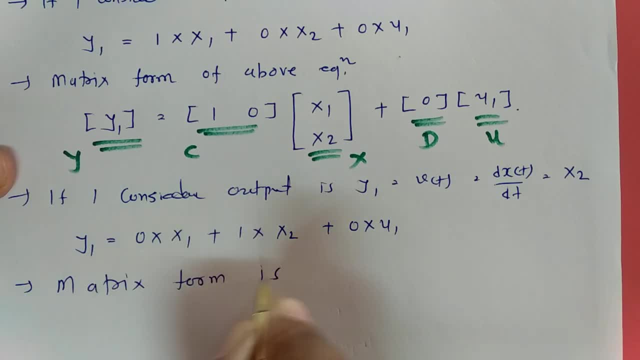 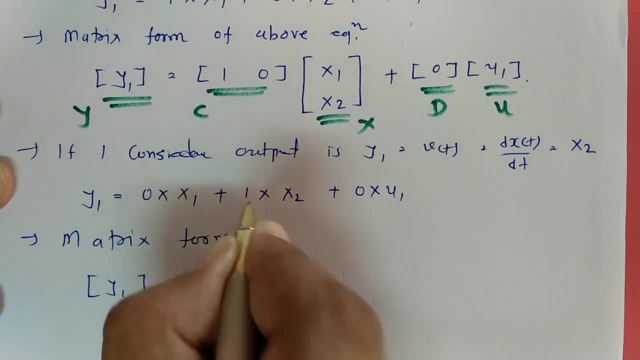 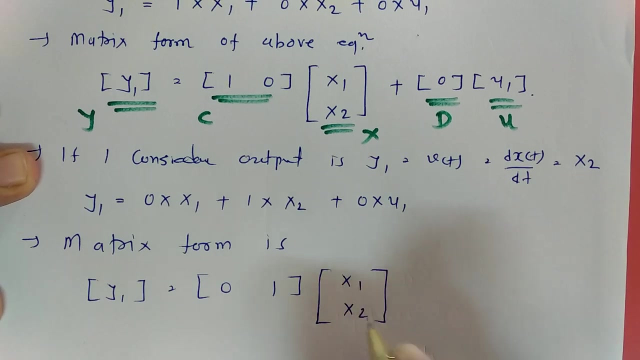 form is: this is y1. this terms are 0 and 1.. So now it is 0 and 1 and this matrix is x1, x2.. So this is what getting multiplied is equal to y1.. So this is y1, x2, x1, x2.. So this: 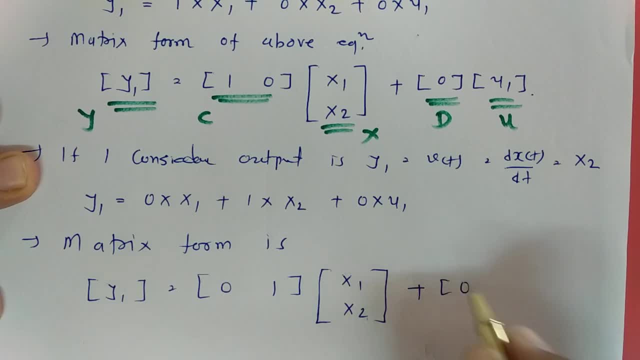 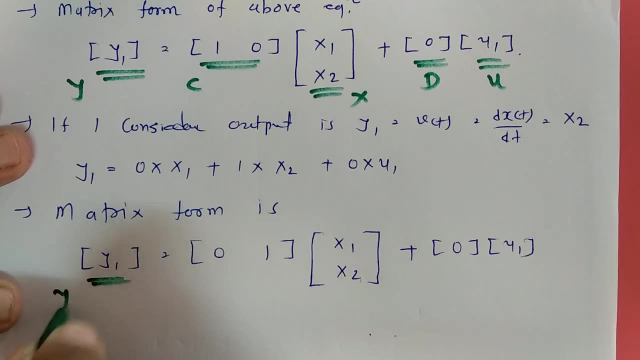 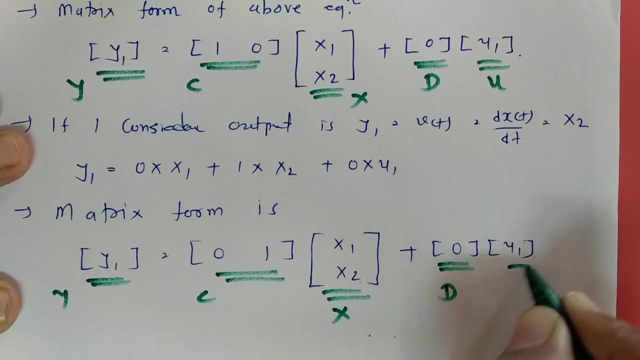 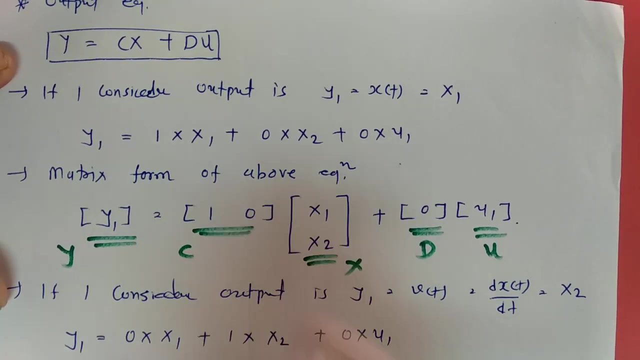 is resulting into this: plus, this matrix is 0 and this matrix is u1., Where one can say: this is output matrix, this is c matrix, this is x matrix, this is d matrix and this is input matrix u. So this is how I can be able to write this output equation, which is what, as 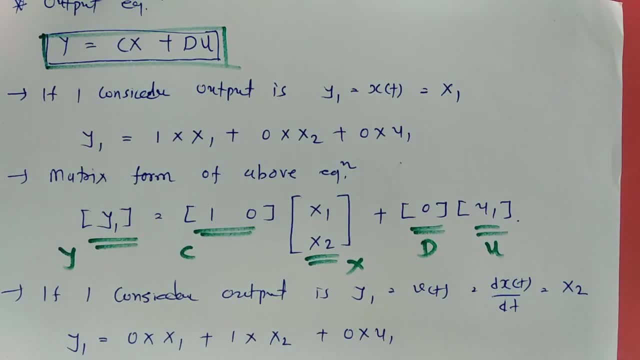 per y is equals to cx plus du. Now let us see how one can do state space analysis, and this state space analysis is very powerful tool in control system engineering where one can have observation and analysis of non-linear time variant system with accuracy, as well as multiple input and multiple output. 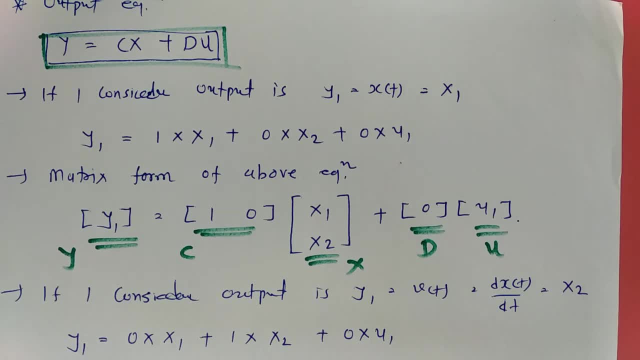 so this is what about mechanical system, state space modeling. So once you understand what is that, which is that, what is mechanical system, one can be able to derive its state-space matrix analysis, and that is very useful to have a derivation. Thank you so much for watching this video. In next video I will be 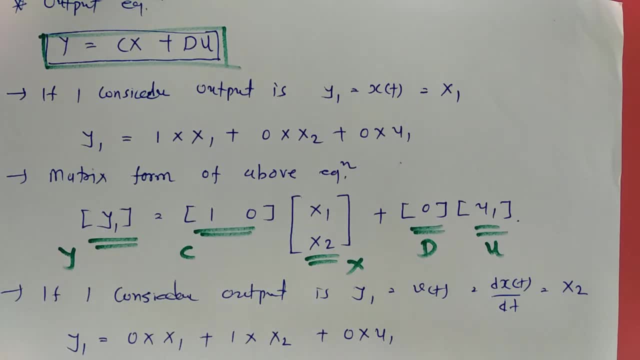 explaining state-space modeling for electrical system. Thank you so much for watching this video. 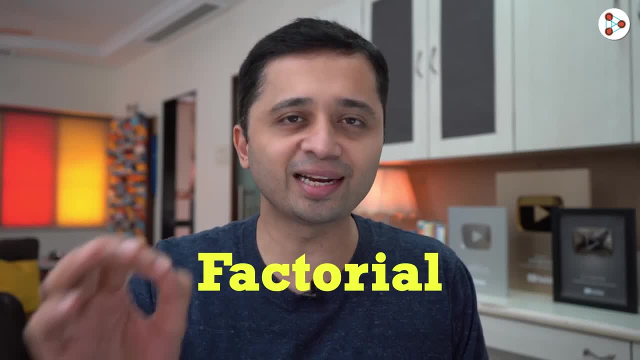 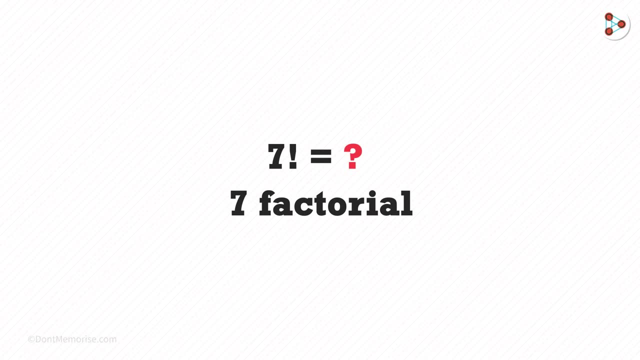 The concept of factorial is very important in mathematics. It's written as an exclamation mark after the number. So if we have this, then we call it 7 factorial. But what is its value? Let's see, Suppose we need to find the value of 3 factorial, We write it as 3. 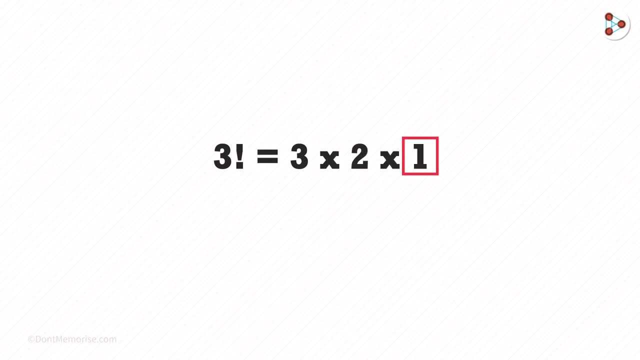 times 2 times 1.. We go on until we reach the number 1.. So the value of 3 times 2 times 1 is 6.. So what will be 5 factorial? It will be 5 times 4 times 3 times 2 times 1, and we 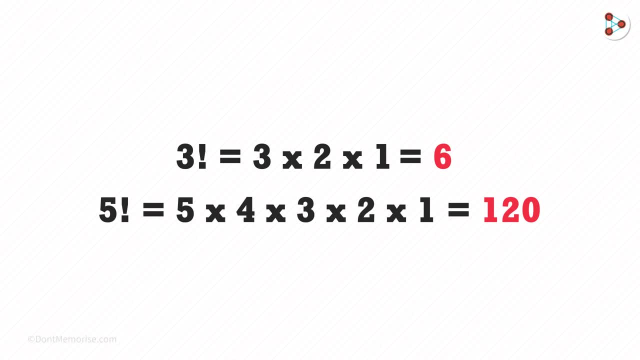 have reached till 1.. So we shall stop. The answer is 120.. Now, before signing off, here are a few interesting questions for you. What is the value of 1 factorial And what is the value of 0 factorial And what is the value of 7 factorial? Do let us know in the comment.